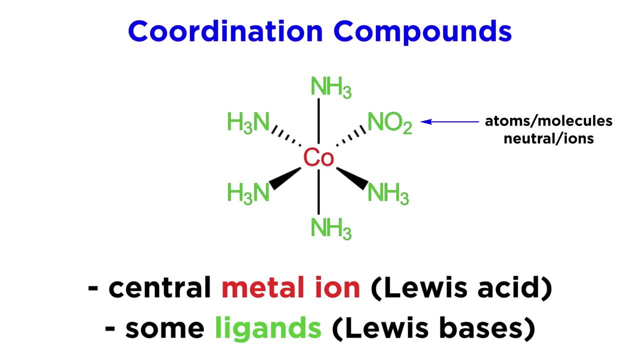 of a metal atom bonding with ligands. As we know, these ligands can be atoms or molecules, either neutral or ions. But we are going to go a lot deeper now in learning about precisely how metal atoms interact with ligands and what kinds of ligands we can expect to see. The first thing we 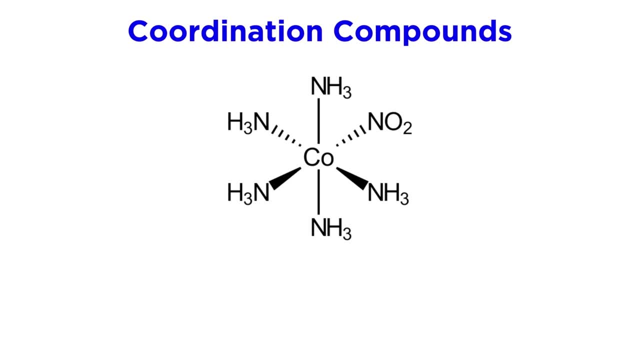 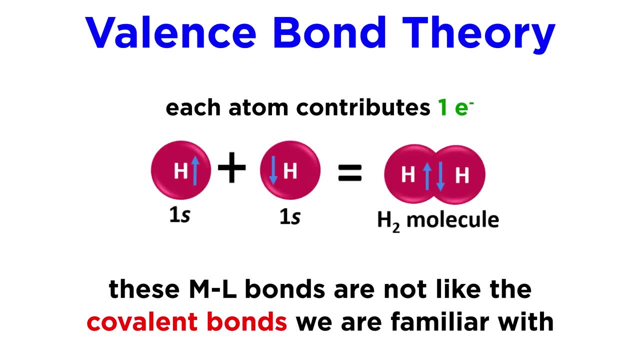 need to discuss is the types of bonds that can occur between a metal and a ligand. One would be tempted to look at the bond between a metal and a ligand as a normal covalent bond, which, as we know, according to valence bond theory, is a situation where each of them contributes one electron. 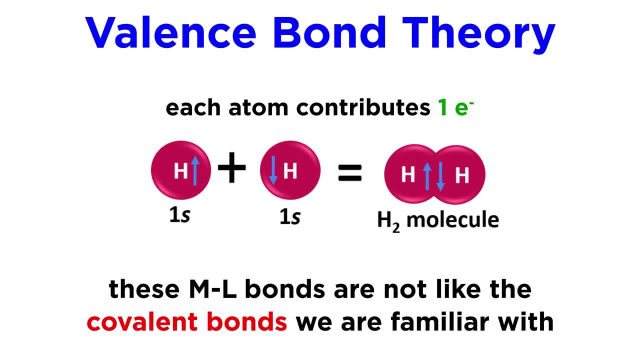 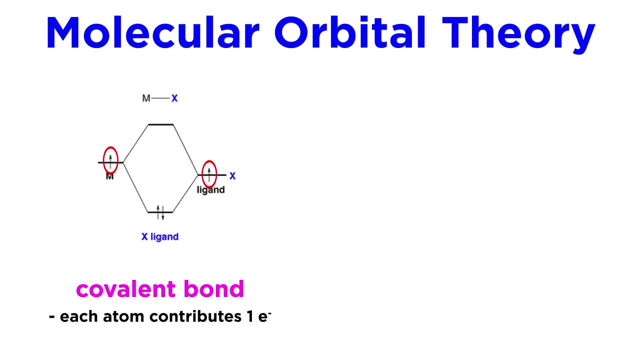 to the bond, and the orbital overlap is what creates the bond. From the perspective of molecular orbital theory, that would look like this: where each contributes one electron, so both of them sit down here in this sigma bonding orbital. However, in most situations, a more accurate description of 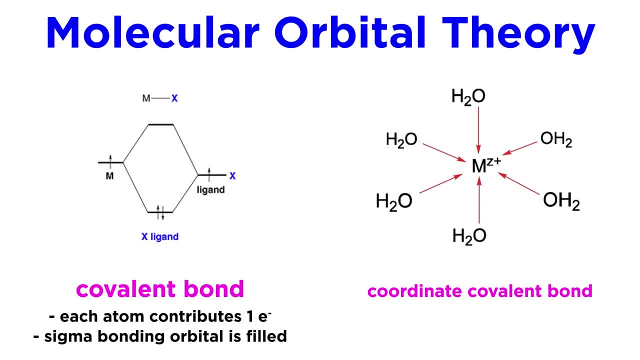 metal-ligand bonding is the coordinate covalent bond or dative bond. In a dative bond, the metal acts as a Lewis acid and the ligand acts as a sigma. In a d-bond, the metal acts as a Lewis acid. 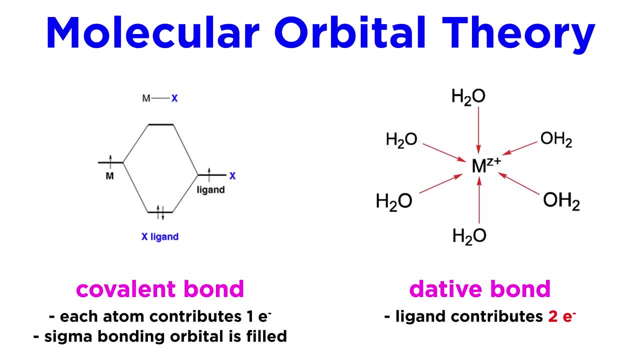 and the ligand acts as a sigma. In a d-bond, the metal acts as a sigma. In a d-bond, the metal acts and the ligand acts as a Lewis base, contributing both electrons to the bond. If using molecular orbital theory, that would look like this, with the ligand usually sitting. 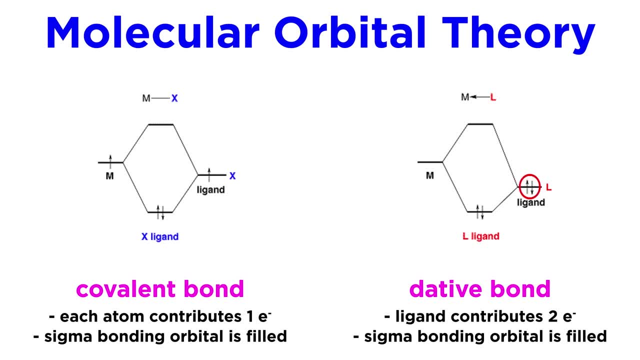 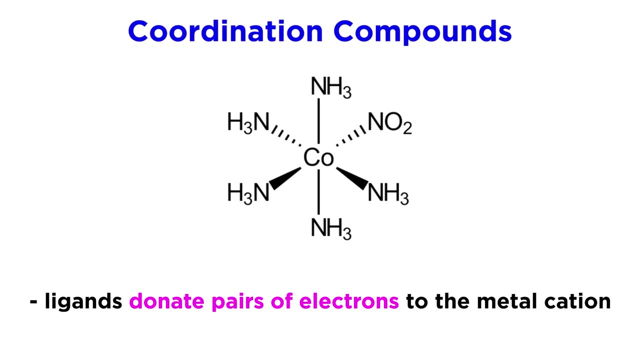 at a lower energy than the metal and contributing both of these electrons to the sigma bonding orbital. This is not really a new concept, as we have seen electron-rich species acting as Lewis bases before. The one thing that we'll take a bit of getting used to is that when we have ligands contributing 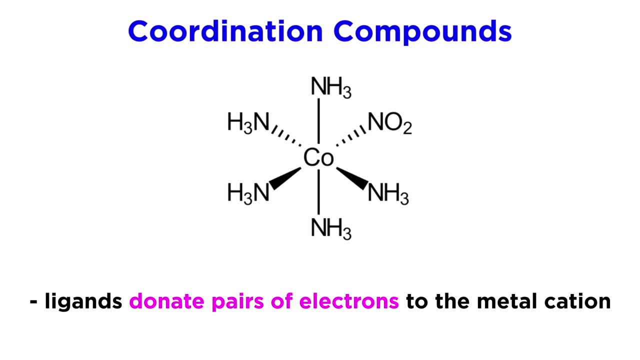 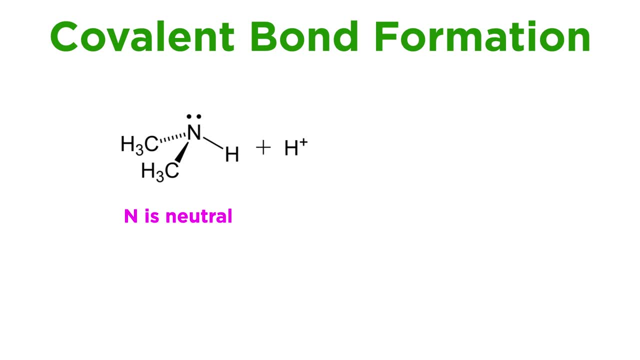 pairs of electrons to form dative bonds with a metal cation, we do not end up with formal charges in the same way we would expect in organic chemistry. In other words, if a nitrogen atom uses its lone pair to pick up a proton, it ends up. 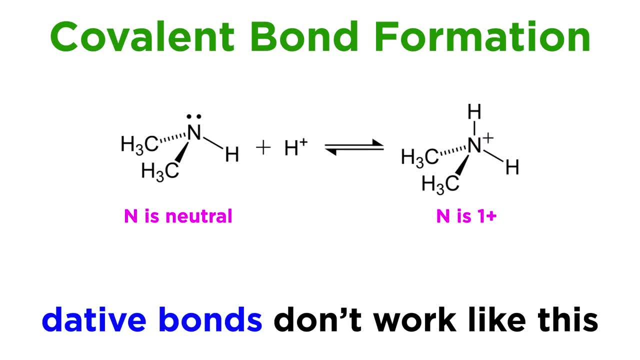 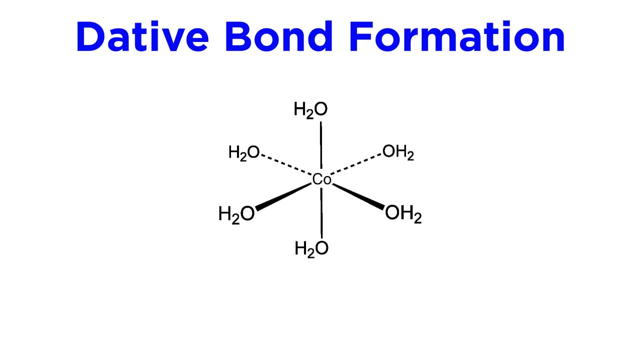 with a formal positive charge. But that will not be the case when neutral ligands use their electron density to coordinate to a metal atom. So, for example, if this cobalt center was coordinated to six water molecules acting as ligands, These oxygen atoms would not have formal positive charges and the whole complex would have. 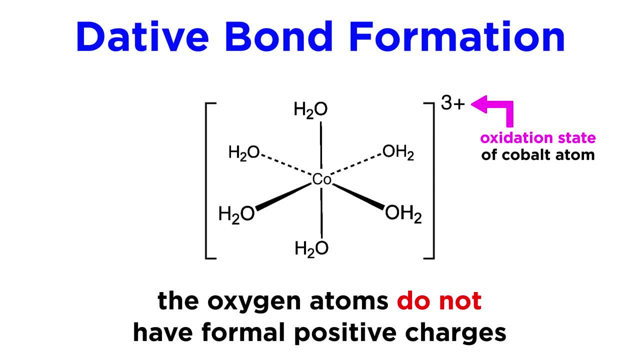 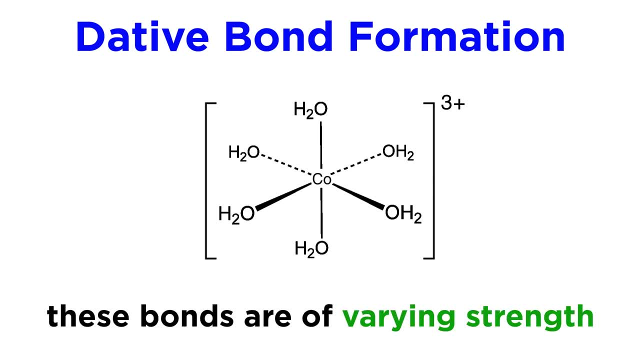 an overall charge of three plus which, by convention, corresponds to the oxidation state of the cobalt atom. These dative bonds are of varying strength. For example, these cobalt-oxygen bonds are particularly long and weak. Many metal ligand bonds are quite weak, in fact, and in such a case we would refer to. 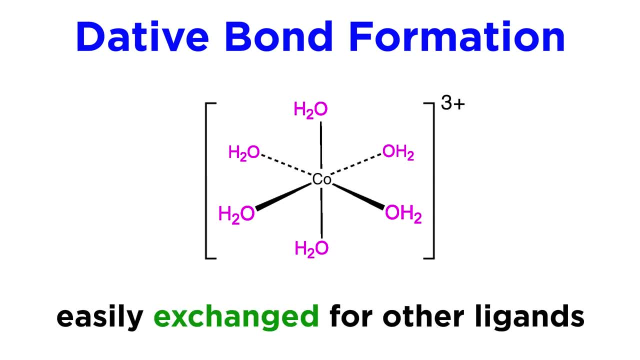 these ligands as ligands. These ligands are known as labile, which means that they are easily exchanged for other ligands that make stronger bonds. Indeed, new ligands displacing existing ligands in a transition metal complex is a very important 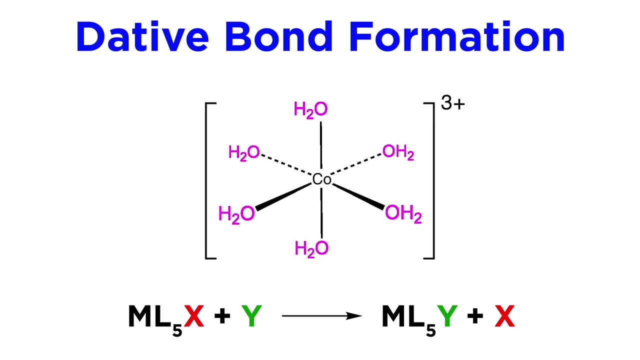 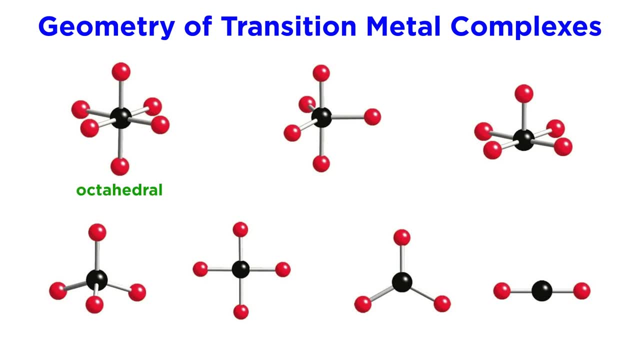 reaction that we will be discussing in great detail later. The geometries of these complexes should already be very familiar from general chemistry. We just saw an example of an octahedral complex. Other geometries include trigonal bipyramids. Other geometries include trigonal bipyramids. 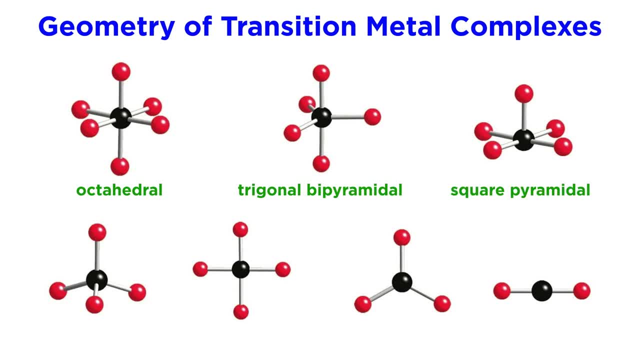 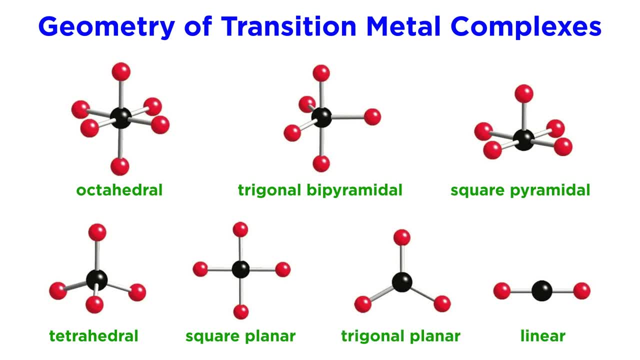 trigonal, planar, linear, essentially all the ones we already know just now, with metals in the center. It will not always be obvious which geometry a complex will take on, as this may depend on the identity of the metal atom as well as the ligands. 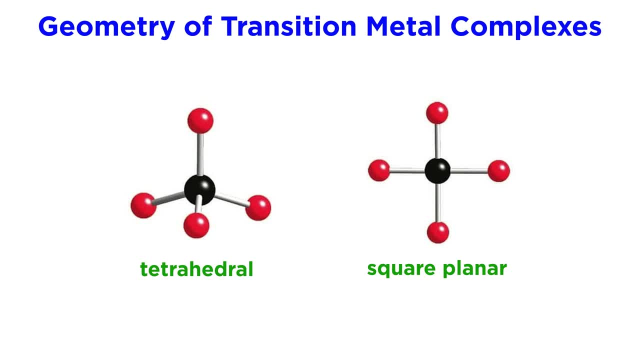 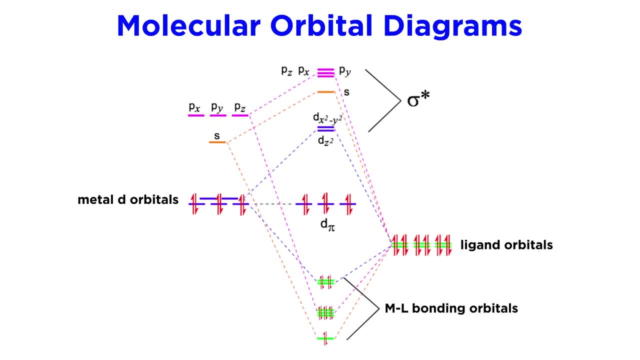 For example, with four ligands, will a complex be tetrahedral or square planar? Answering this question will require attention, require a tutorial all to itself, but one thing that we should look at briefly right now is a molecular orbital diagram for transition metal complexes. 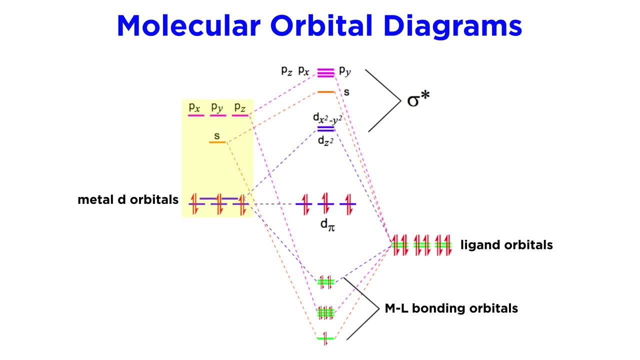 On the most basic level. we simply have to understand that on the left, we have the orbitals from the metal, the lowest energy often being the d orbitals. then higher up is the s orbital and then the p orbitals. On the right, we have the orbitals from the ligands, which tend to be lower energy than 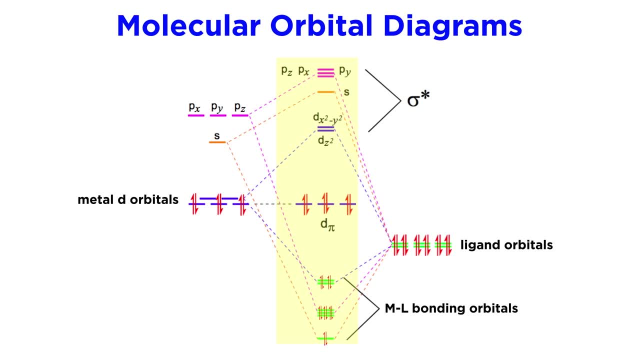 those of the metal. When these combine we get the molecular orbitals in the center. Down low we have the M-L bonding orbitals. These get filled first with the electrons donated by the ligands. Then we have the d pi orbitals which will hold the metal's d electrons. so these constitute 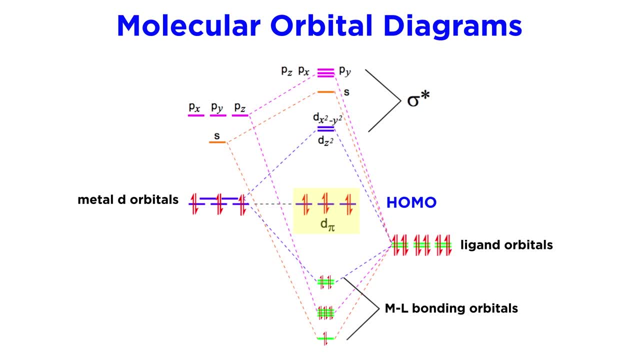 the highest occupied molecular orbitals, or HOMO. Then, above that, we have the unoccupied molecular orbitals, starting with the remaining d orbitals. This dz squared orbital is the most important orbital of the metal. This d z squared orbital is the highest occupied molecular orbital, or HOMO. 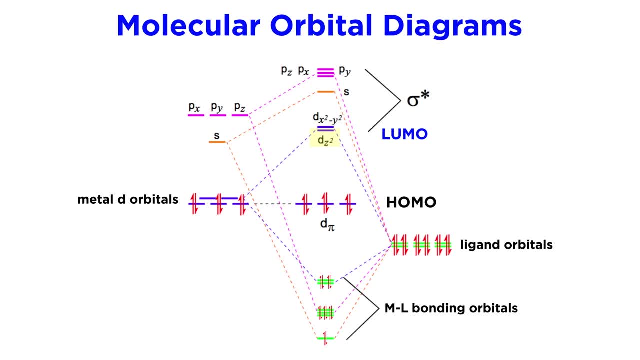 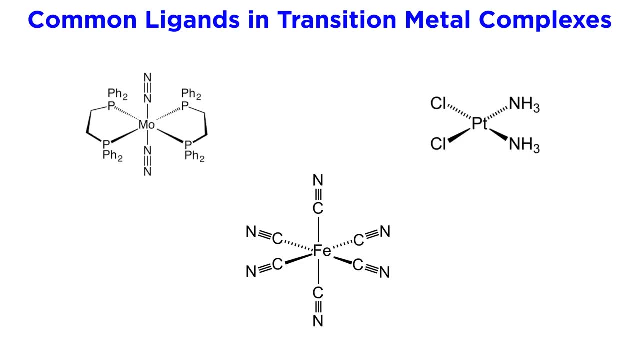 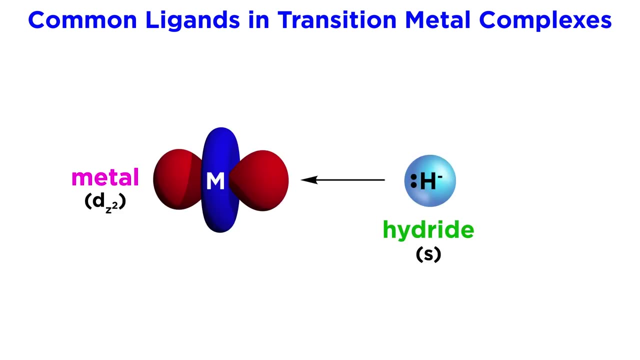 This orbital tends to be the lowest unoccupied molecular orbital, or LUMO, so we will frequently see incoming ligands interacting with this orbital. Speaking of ligands, let's now become familiar with some common ligands and describe how they bond to the metal atom. 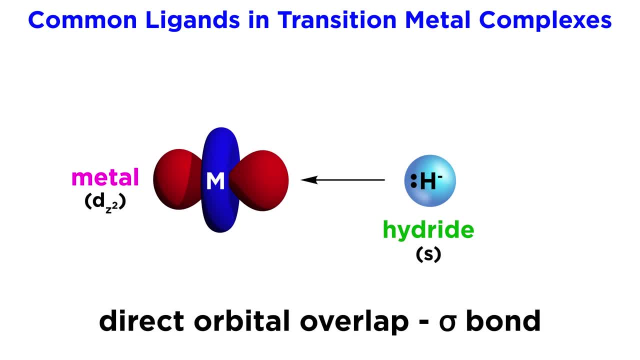 First up the hydride ion with its pair of electrons. Its lone s orbital will overlap directly with some orbital on the metal, as in this case with the dz squared orbital, to produce a sigma bond. The halide ions will all behave this way as well, though these have four pairs of valence. 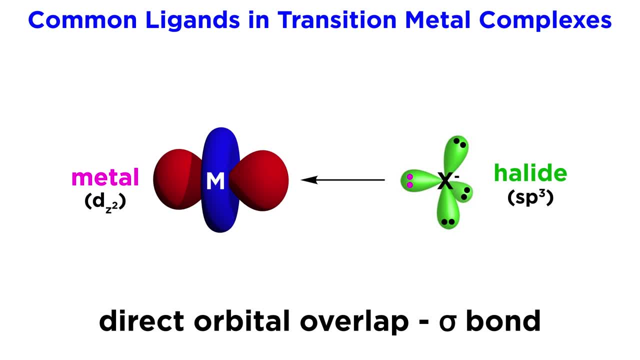 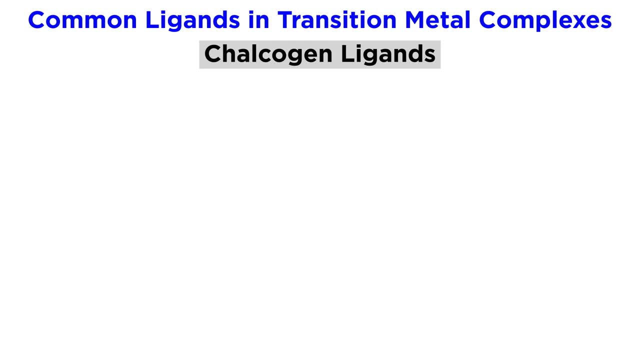 electrons and are sp3 hybridized. One of these lone pairs will be donated to form the dative bond. Now, from the halogens we move to the chalcogen ligands. Oxide and sulfide ions, which each have four lone pairs, can both act as ligands and they 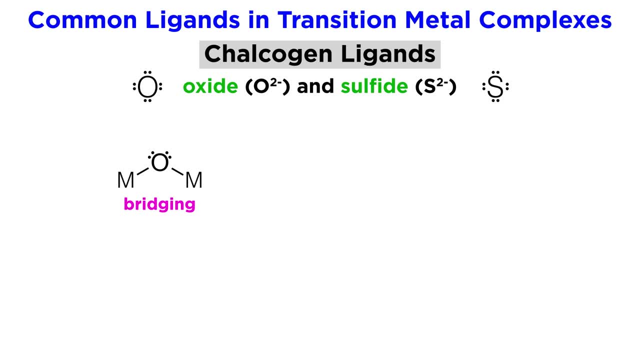 can do so from either a bridging position, where they make two bonds to two ligands, or, in the same position, where they start to form a bond bonds to two different metal atoms, or a terminal position, where they make two bonds to the. 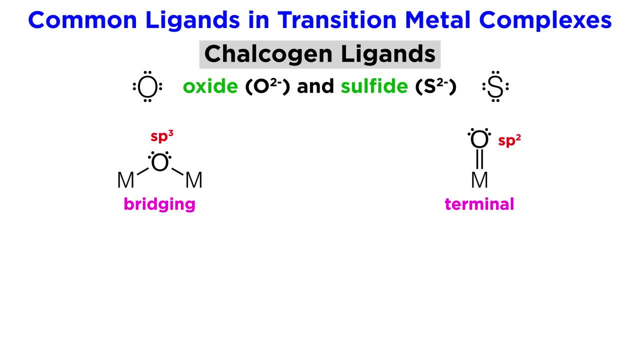 same metal atom. Oxygens in these positions would be sp3 and sp2, hybridized respectively. as we would expect, In the bridging scenario, the electron pairs are donated into the dz-squared orbitals of two different metal atoms, whereas in the terminal scenario the first bond a sigma. 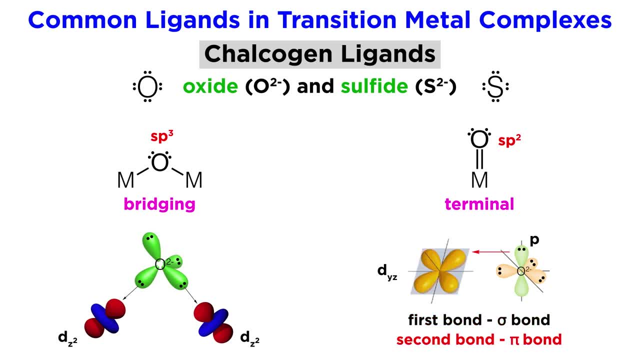 bond is oriented this way as well, while the second bond, a pi bond, occurs due to overlap of the unhybridized p orbital on the oxide with the dyz orbital on the metal. This is essentially a double dative bond. Alkoxides and sulfoxides, which each have three lone pairs, behave in the same manner. 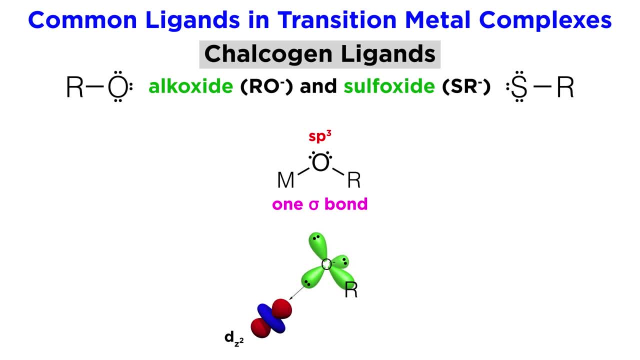 although they tend to only donate one pair of electrons to make the sigma bond with one metal atom. The same can be said for ethers and sulfides, as well as water, which each have two lone pairs. These can donate one pair of electrons to a metal atom to form a sigma bond. 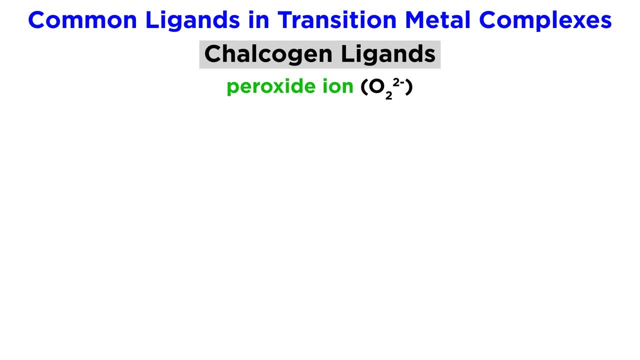 There are some more interesting ligands involving oxygen, such as the peroxide ion. This has a two minus charge and the highest occupied molecular orbital is a pi star orbital. so this ligand can bond with two metal atoms, one per oxygen. 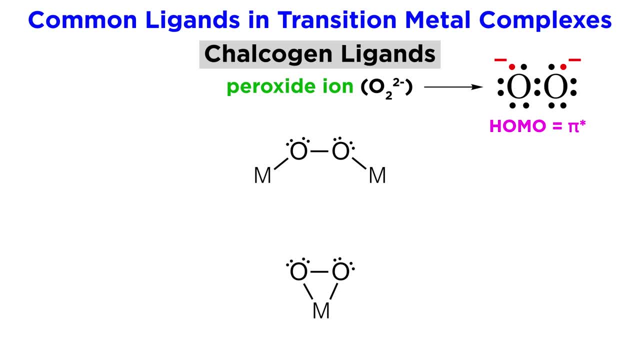 Therefore both oxygens can bond with the same metal atom. A similar ligand is the superoxide ion. This has just a one minus charge because one of the oxygens is a radical. The one with the full octet will do the coordinating again from the pi star orbital. so this ligand 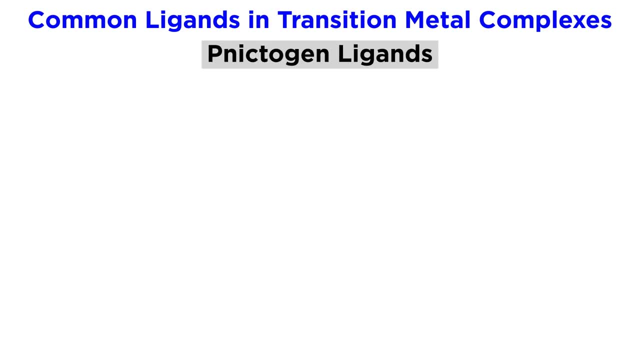 will typically bond to just one metal atom. Moving on to nictogens, there are a number of nitrogenous ligands. The nitride ion has a three minus charge. The nitride ion has a three minus charge, The nitride ion has a three minus charge, and thus four lone pairs. 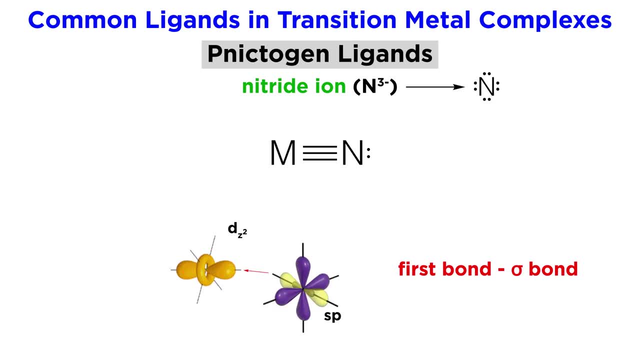 Three bonds can be made to a metal atom, one of which- a sigma bond- will occur between the sp-hybrid orbital on nitrogen and the dz-squared orbital on the metal, and the other two are pi bonds between the two unhybridized p orbitals on nitrogen and the dxz and dyz. 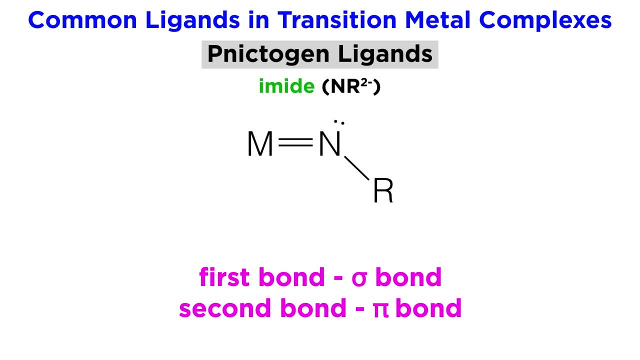 orbitals on the metal. Imides, or nr two minus, can do something similar just with one sigma bond and one pi bond. Amide and phosphide ions, or nr two minus and p-r two minus can make one sigma bond. 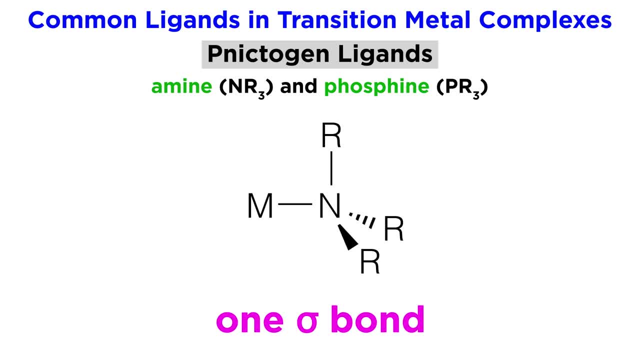 to a metal atom, as can neutral amines and phosphenes. Finally, the nitrocyl ion, or NO plus, can also act as a ligand. This is an oxygen and nitrogen with a triple bond between them, each having a lone pair. 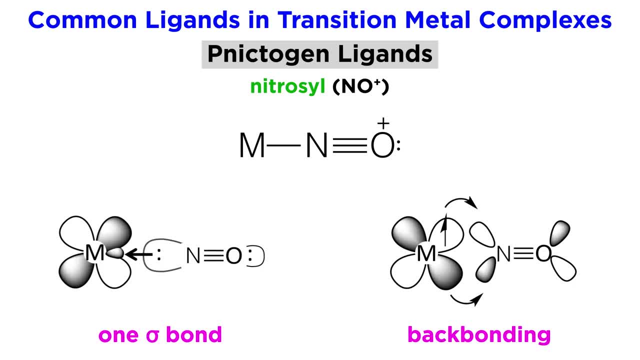 and a formal positive charge on the oxygen. With this we introduce the ligand. We introduce a new concept, that of backbonding from the metal. With this ligand, a sigma bond forms due to the overlap of the two p-sigma orbital from. 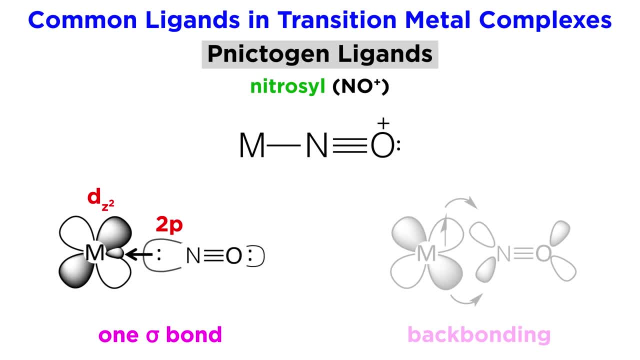 this nitrogen atom and the dz-squared orbital on the metal. And then an additional interaction occurs where the metal donates a pair of electrons from one of its d orbitals into the p-pi-star orbital of the nitrogen. So the nitrocyl ion will be a good ligand for metals that have electrons in these d-orbitals. 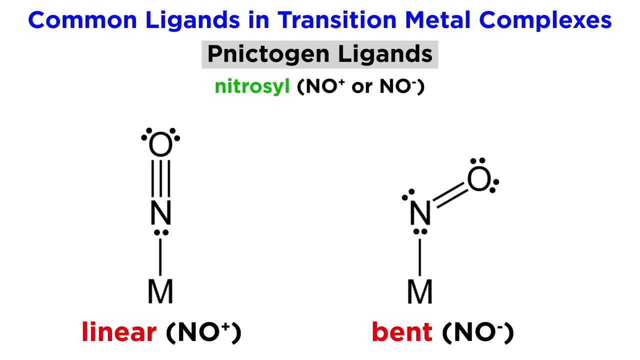 with which to provide this backbonding effect. We should also note that, apart from this linear bonding for the nitrocyl cation, the nitrocyl anion can also coordinate, but in bent fashion, as is shown here. The number of electrons contributed will not change, but we must be aware of this discrepancy. 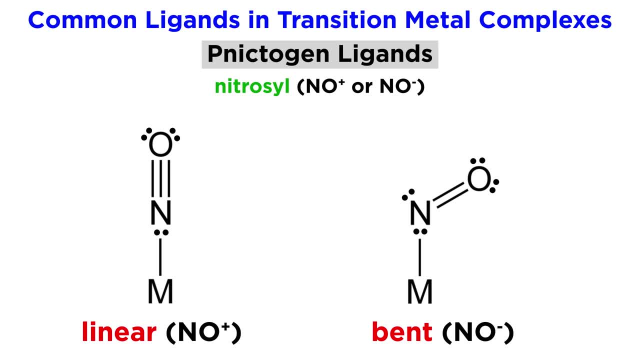 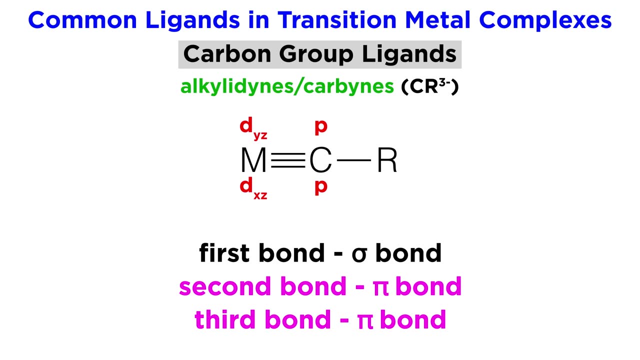 in charge, as well as geometry. Continuing to ligands from the carbon group, first we have alkylidines, or Cr3-. This will be similar to the nitride, where we get a sigma bond, as usual, and then two pi bonds between the p orbitals on carbon and the dxz and dyz orbitals on the metal. 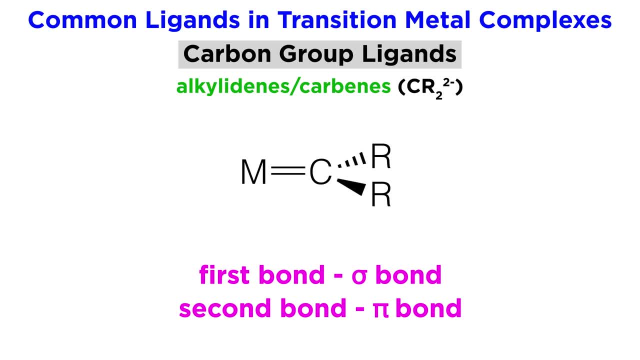 Then alkylidines or Cr2- will form a sigma bond and one pi bond. Carban ions will donate the one lone pair to form a sigma bond, as will analogous ligands replacing carbon with silicon, germanium or carbon. 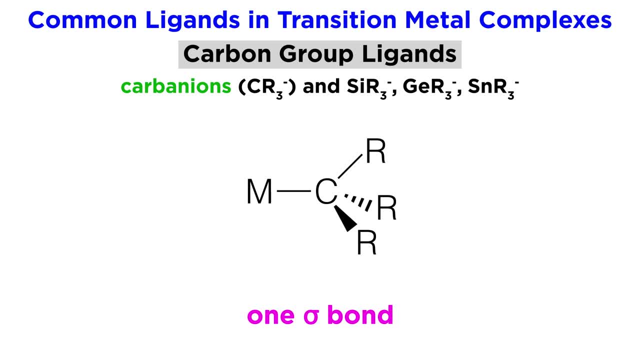 So we get a sigma bond and one pi bond. Then, finally, an extremely common ligand will be the carbonyl or CO ligand. When encountered in this form, it will look like this, with a triple bond between the atoms and a lone pair on each. 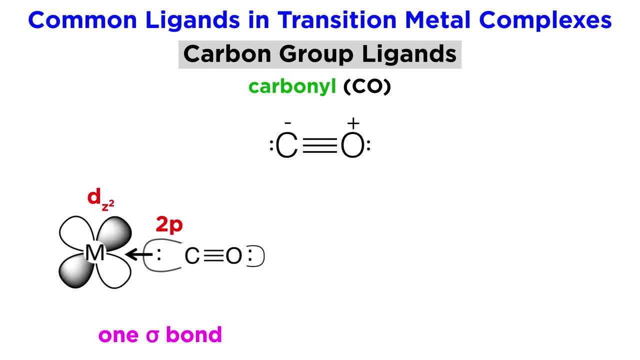 This will work very similarly to the nitrocyl ion. The carbon donates its lone pair in the 2p sigma orbital to generate the sigma bond, and then the 2p pi star orbital on the carbon accepts backbonding from one of the d orbitals. 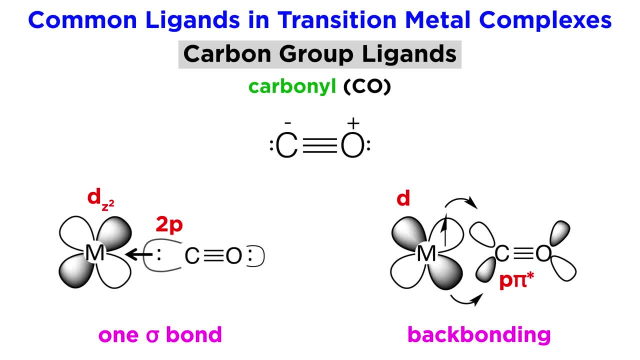 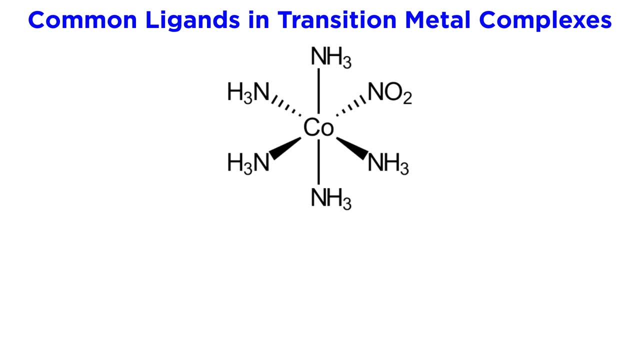 and then the 2p pi star orbital in the metal. When this type of backbonding is present, the ligand is bound quite strongly to the metal. So that covers the general concept of bonding in transition metal complexes. We have learned about dative bonds and how they differ from the covalent bonds we are 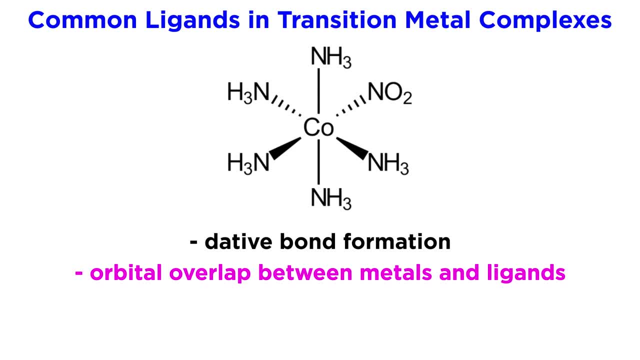 used to the types of orbital overlap that occur between metals and ligands, including the new concept of backbonding, as well as a brief survey of simple and common ligands based on elements from groups 14 and 15.. So let's get started. 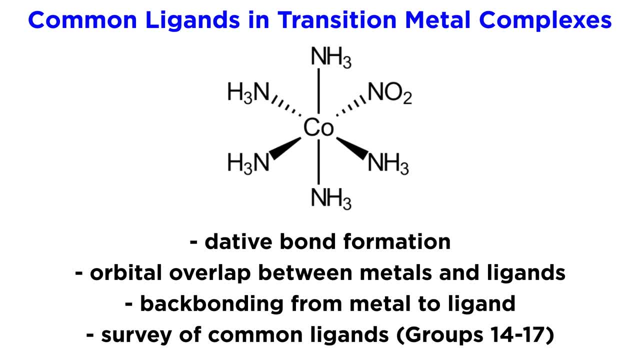 Now let's move forward and check out some trickier ligands.